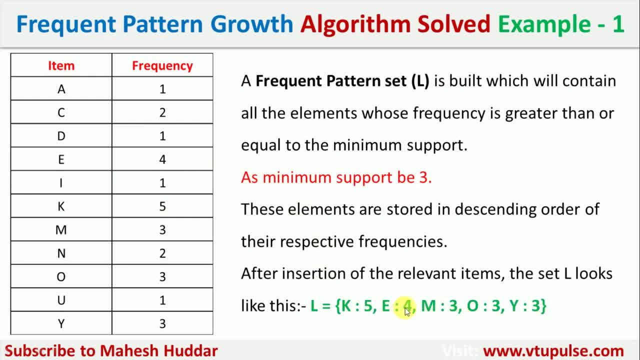 So first K will come and then E will come. M, O and Y were having the same frequency, But M was bought first, and then O and then Y. So that is the reason. This is the order in which we need to keep it over here. 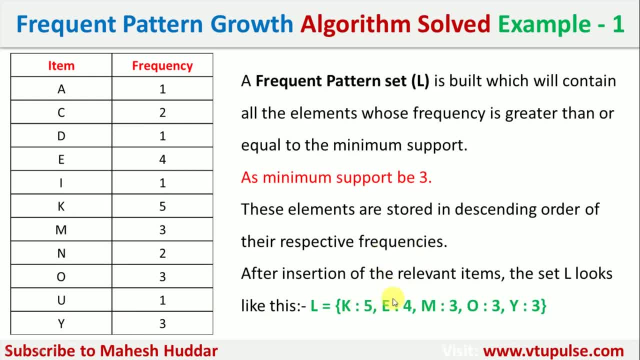 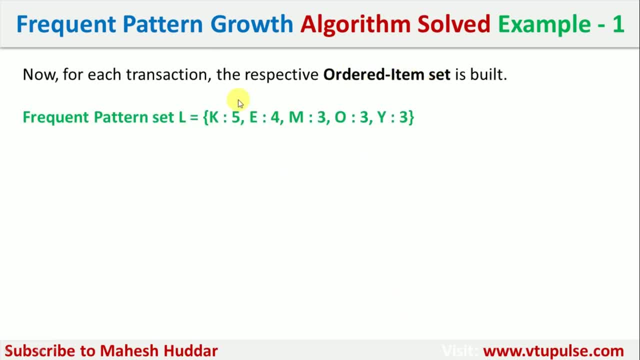 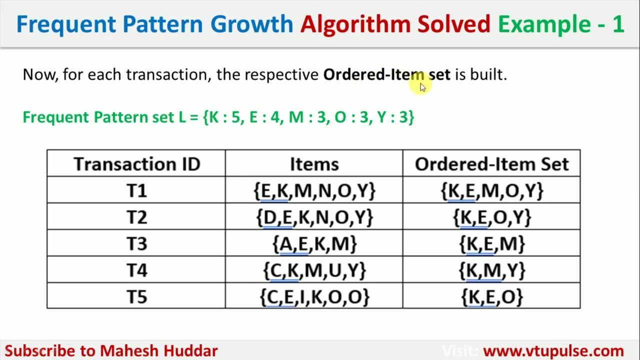 Now, once you find this particular frequent pattern set, that is L- Next, what we need to do is to identify the ordered item sets. So this is a frequent item set, a frequent pattern set we found in the previous step. Using this, we try to find out the ordered item set. 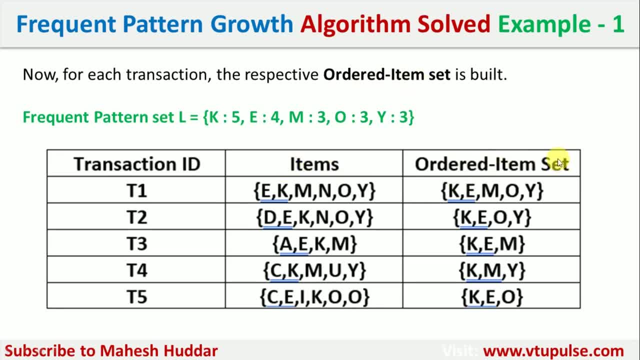 So these are the items. These are the ordered item set. So how to find out is: first we need to check which all items are ordered. These items were present in the frequent pattern set and we need to arrange them in the decreasing order. 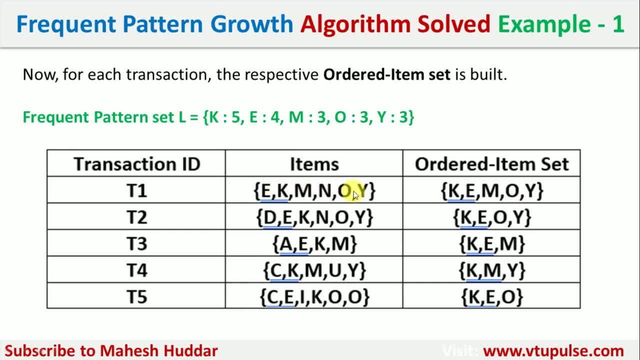 That's it. For example, E is present, K is present, M is present, O is present and Y is present, N is not present. So these items should be kept in the decreasing order. So K will come first, because its frequency is five, and then E, M, O, Y. 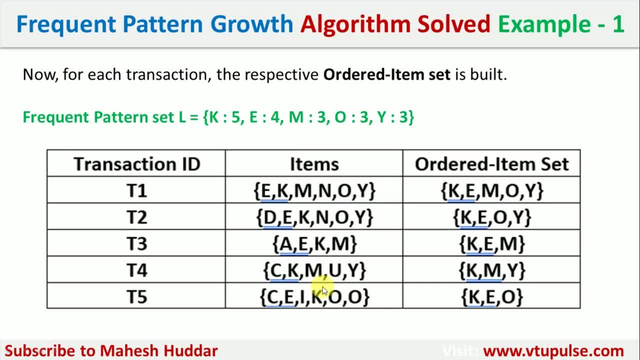 This is the ordered item set. The same thing is repeated for the remaining transactions. For example transaction number four, In this case C, is not present in the frequent pattern set, And then U is not present, K, M, Y is present. 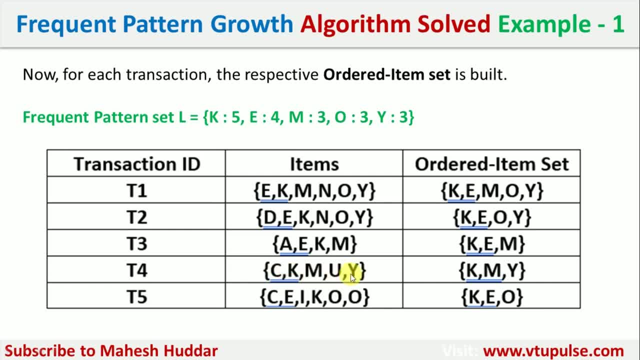 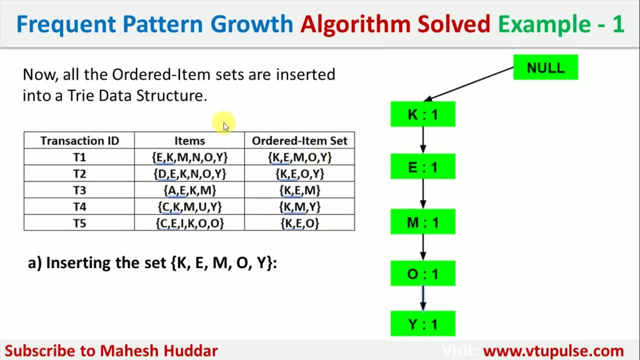 So K is having frequency five, So it will come first and then M and then Y over here. So once you identify the ordered item sets, the next step is to build the tri data structure, which is built something like this: We will start with the null node and for every transaction's ordered item set we will create a path here. 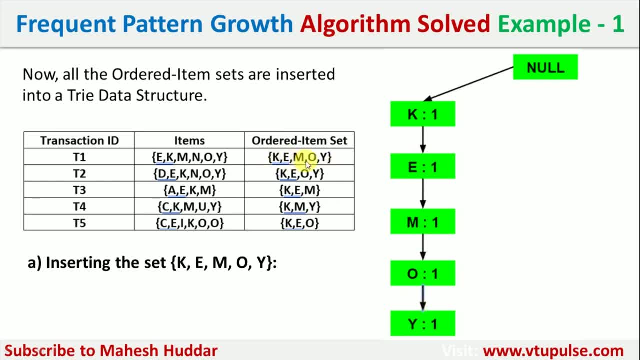 For example, the first one is K E M O Y. So for every node or for every item, we will create one node and initially we assign the frequency as one. here, K is the first node, E is the second one, M is the third one, O is the next one and then Y is the last one. 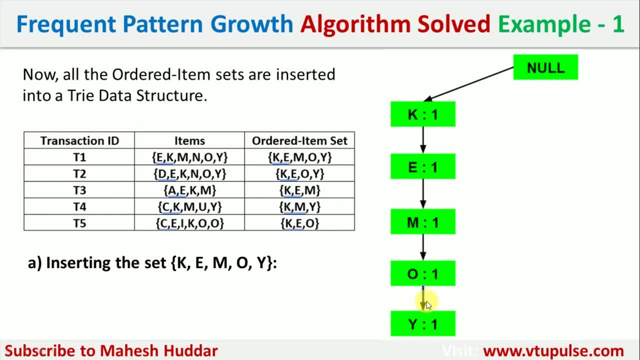 So the frequency of every node is one one. in this case. The second transaction is K E O Y. So if you look at this particular thing, K? E is present and from E there is no direct path for O here. 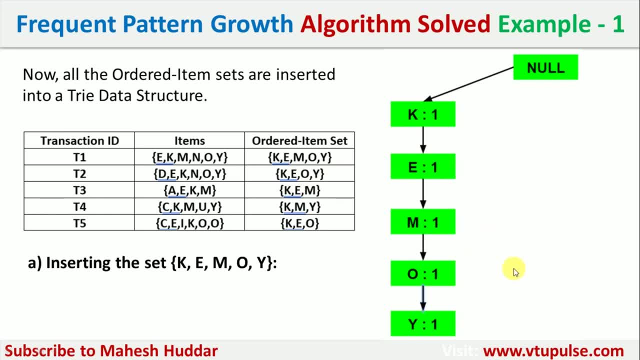 So we need to add one more node here, that is O, and then we need to add one more node, that is Y. K and E were visited one more time, So the frequency will be incremented by one one, and we will add O and Y as the two more nodes in this case. 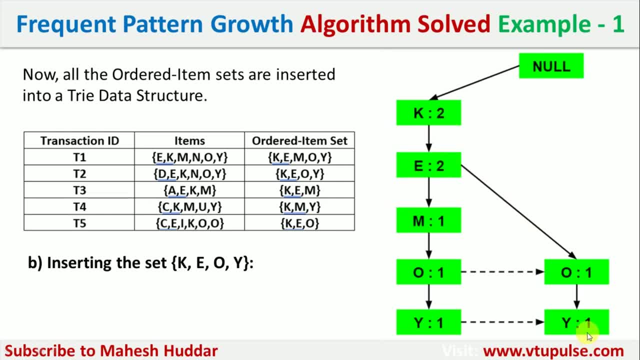 So the frequency of these two is two, two, and this is one one here. The next one is K E M, So K? E will be visited again, M is visited again, So it will become three, three, two in this case. 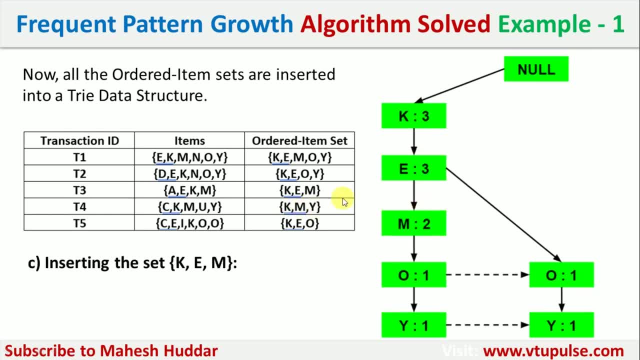 So that is the next thing: K, M, Y, So K. there is no direct path. There is no direct path for M, So it will be four, M will be added here and then Y will be added here. So M will be one and Y will be one here. 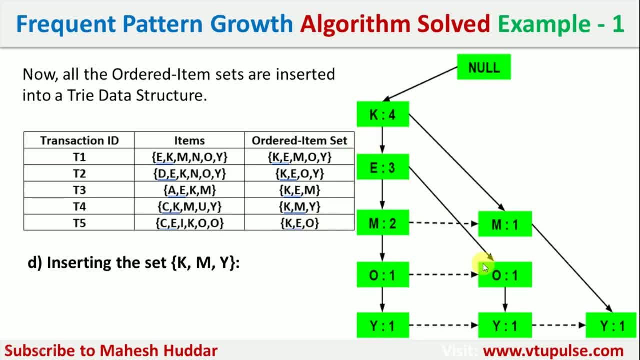 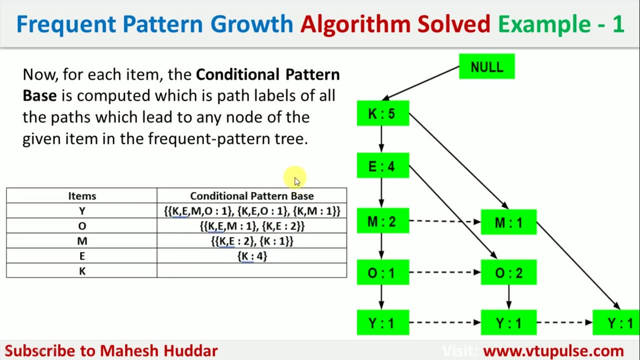 And then the last one is K E O K E O. there is a direct path, So it will become five, four, and then this is two here, So this is the last the transaction inserted here. Once you do this step, the next step is to identify the conditional pattern basis. 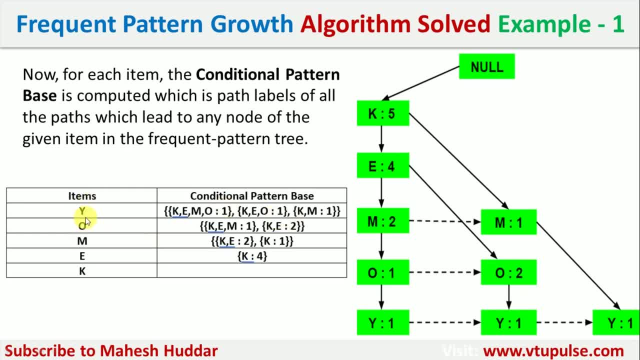 So conditional pattern base for every node we need to identify or every item we need to identify, That is, Y, O M E K. These are the items we have written in the ascending order here. For Y, what are the conditional pattern base? 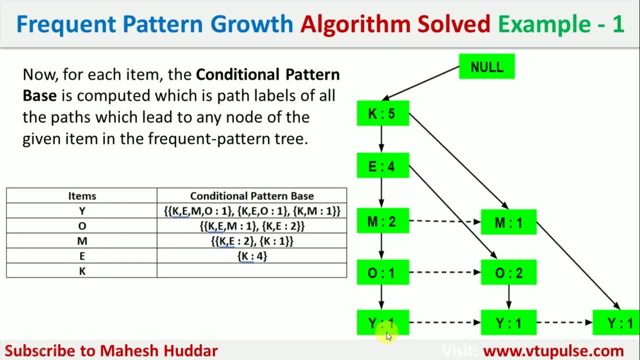 That is nothing but the path to reach that particular Y. So, to reach this particular Y, there are three paths. are there? K E M O, that is the first one. K E O, that is the second one. K M is the next one. 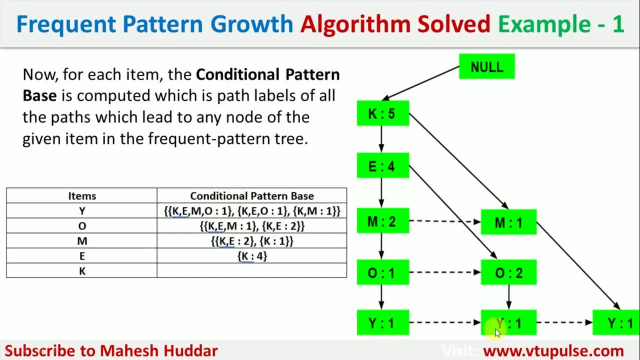 And we need to write the frequency. What is this frequency? So what is the frequency of this particular Y? So in every case one is present, So we write one here. So these are all the conditional pattern basis for Y. here, Similarly for O, there are two paths to reach O. 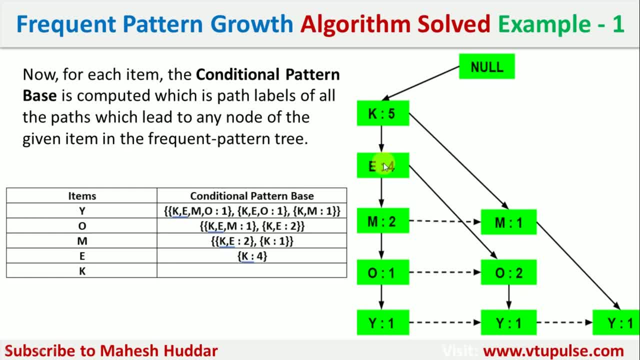 K E, M and then K? E. These are the two things. If I follow this particular thing, the frequency is one. If I follow this path, the frequency is two. For the next one, that is M, we have only one path. 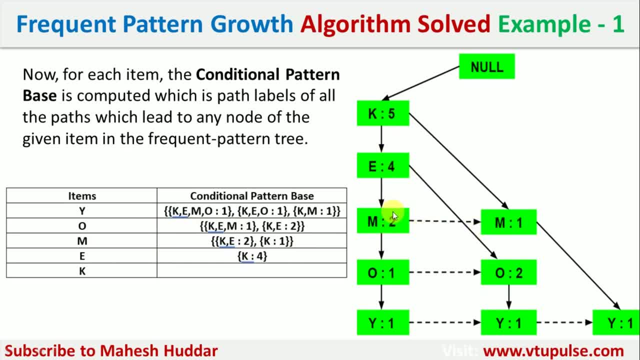 There are two paths again. There is one, and this is the second one, K E 2.. K 1 here, And if you want to reach E, there is only one path, that is K and the value is 4.. 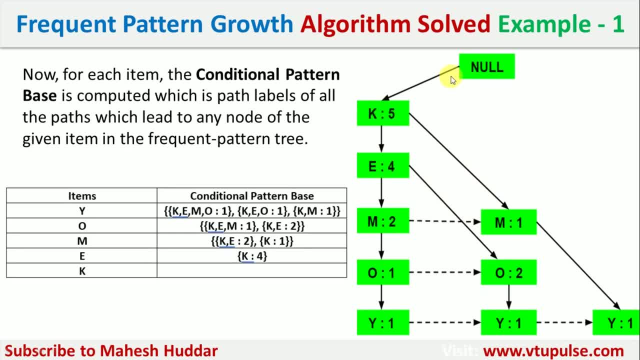 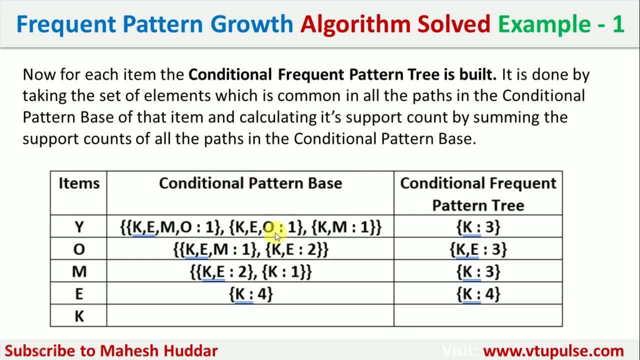 If you want to reach K, there is no node present before this, because there is a null in this case. So these are the conditional pattern basis. Once you find the conditional pattern basis, we need to find out the conditional pattern tree here, That is, conditional frequent pattern tree. 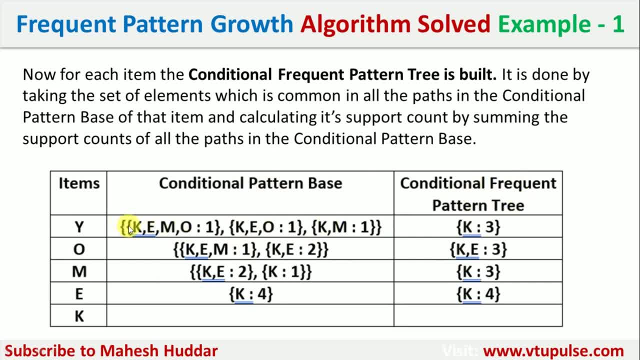 So how it is identified is we need to check the common element or elements from this conditional pattern basis. So in this case, K is the common over here, So K will come here and we need to add the frequency, That is 1, 1, 1.. 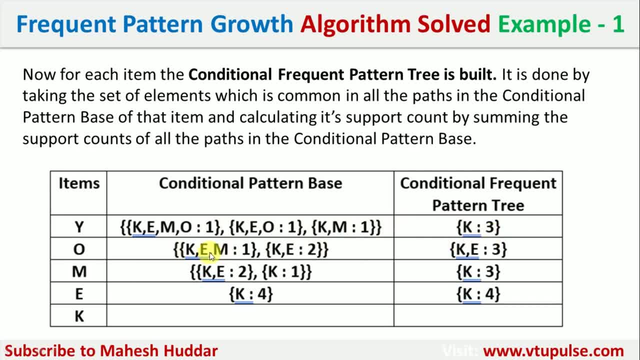 It will become 3 here. In the second case K E is common, So K E will come here and the frequency will become 3 in this case. The third case: only K is common and the frequency is 2 plus 1.. 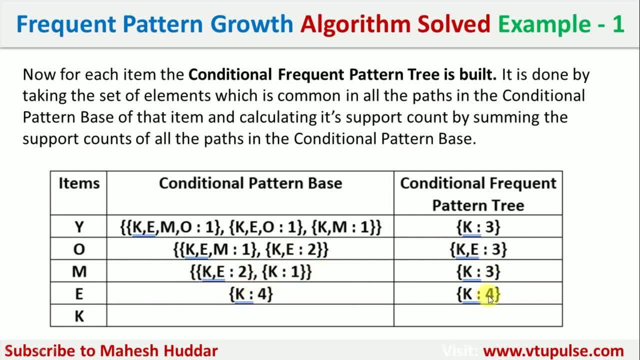 That is 3.. In the next case, K is the only element, So K 4 will be nothing. For the last one, K, there is no path. in this case We found the conditional frequent pattern trees. Using this particular tree we can write the frequent pattern rules. 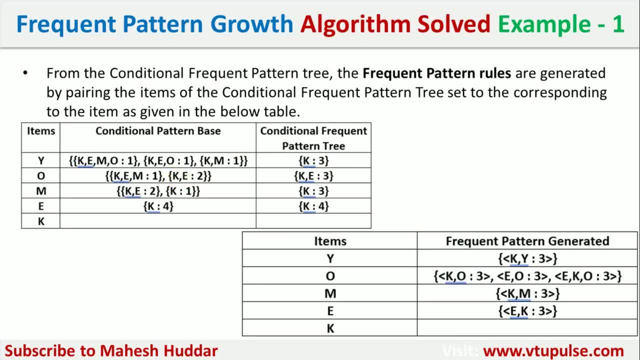 So how can we write the frequent patterns is: Look at this particular thing. The item is Y and the conditional frequent pattern is K in this case. So the rule can be K: Y and its frequency K Y, 3 here. 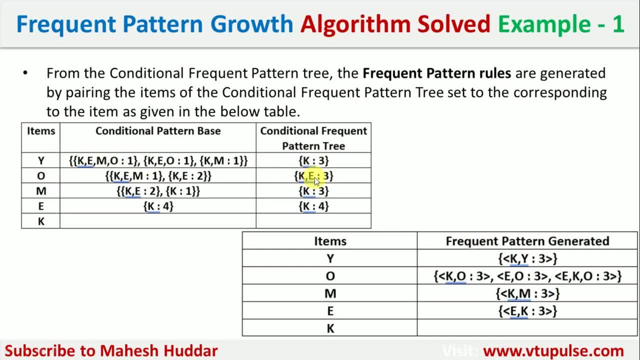 Similarly, item is O and the conditional frequent pattern tree is K? E. So K? O is the one rule, E O is the second one, K E O is the third one. In every case we need to write 3 as the frequency. 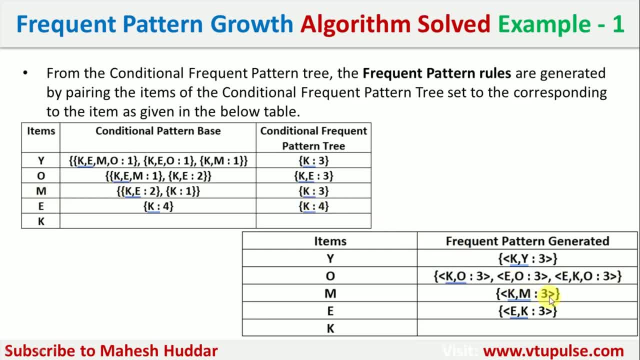 The next one is K M. That is the only possibility and its frequency is 3.. K E is the last possibility and its frequency is 4.. Actually, we have to write 4 here Now. this is how frequent patterns are generated. 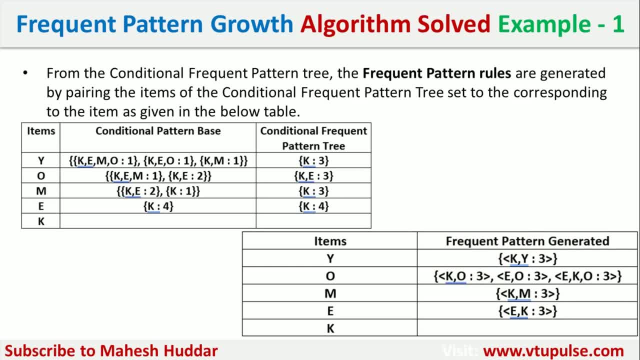 Once the frequent patterns are generated, the last step is to write the rules in this case. So how to write the rules is: consider one frequent pattern and then try to write the rules, All possible rules. you can say K, Y. What is the possible rule in this case?